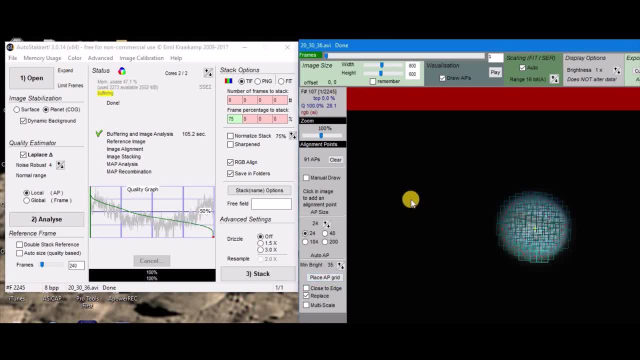 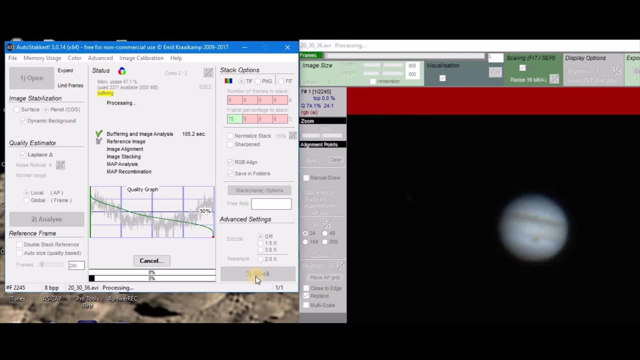 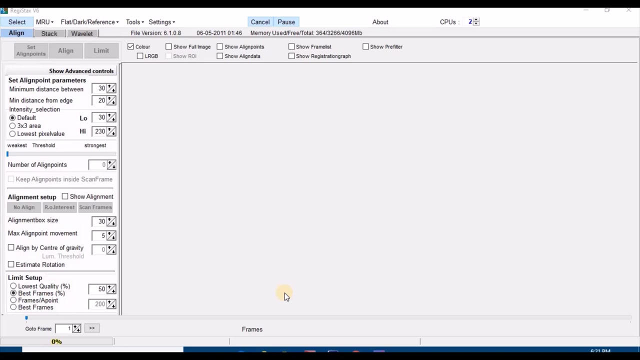 And we also have a moon here, so you want to select this moon and then click stack. This will take several minutes to stack, so I'm going to pause the video and we'll come back with Registax. Okay, now that AutoStacker is done stacking, you want to open up Registax 6 and 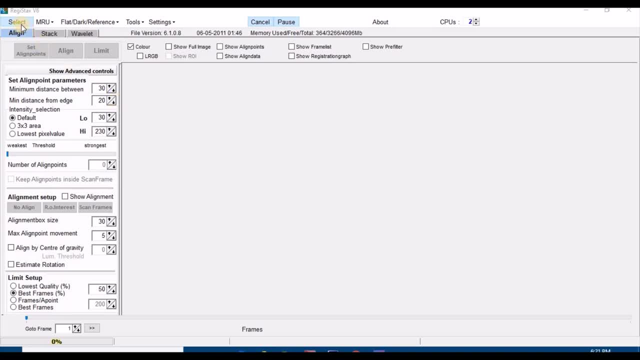 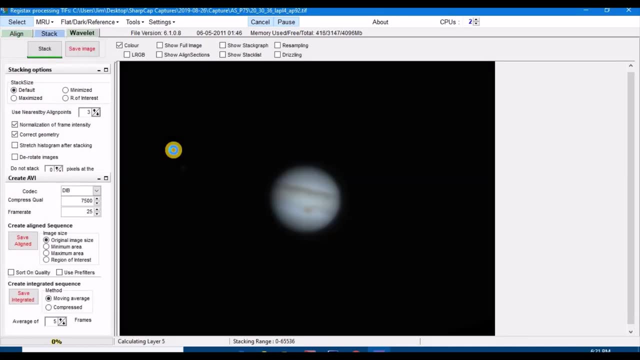 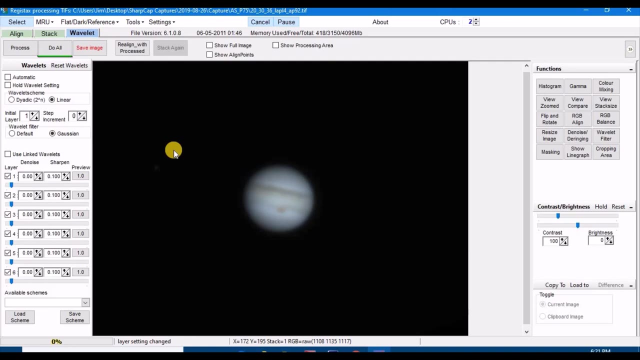 click on select And bring your stacked image into Registax. The first thing you want to do is you want to sharpen this image, So I'd like to use the first and six layers for sharpening. I'm going to take that slider all the way up. 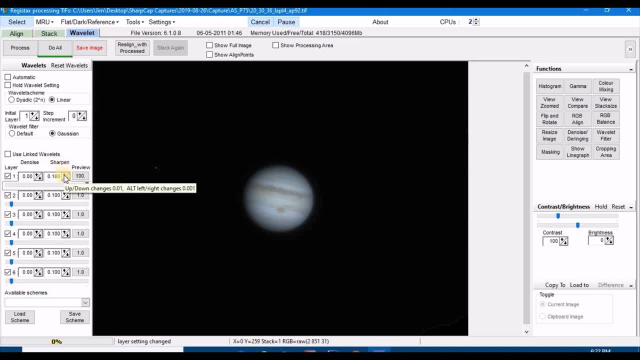 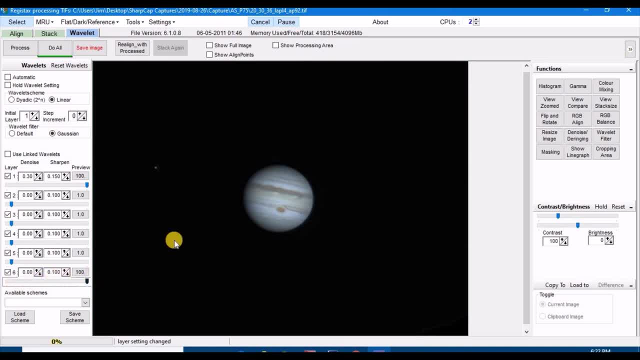 And then I want to take this number six slider and slide it all the way up, And then I want to take this number six slider and slide it all the way up, And that gives you a pretty sharp image. So now you want to go to your histogram over here. 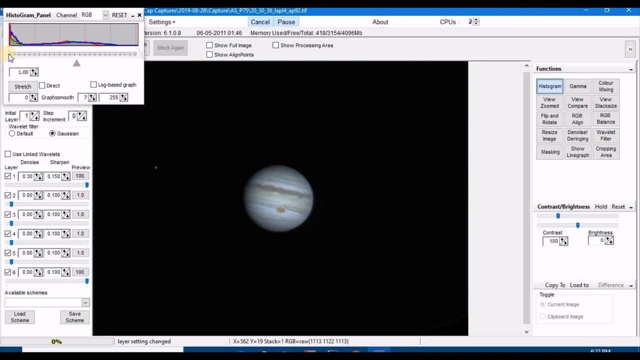 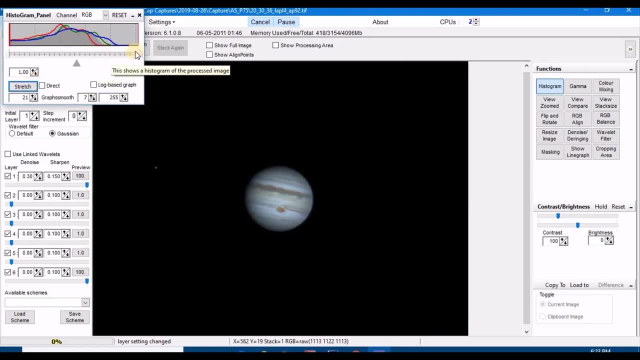 I'm going to stretch this histogram And stretch it to right there, Click stretch And then we're going to stretch it back to lighten it up a little bit more. And then we're going to stretch it back to lighten it up a little bit more. 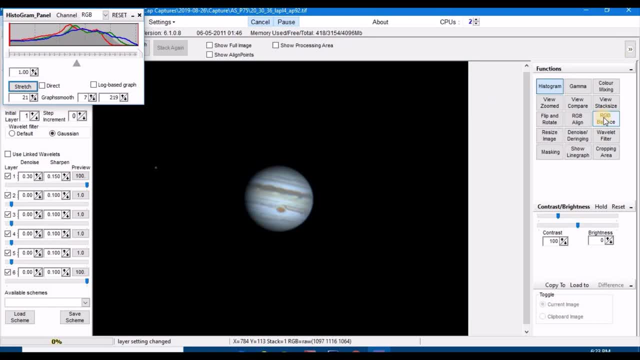 And now you can see these are all the way up. And now you can see these are all the way up And you can see these are not balanced And you can see these are not balanced. So we need to click RGB balance. So we need to click RGB balance.